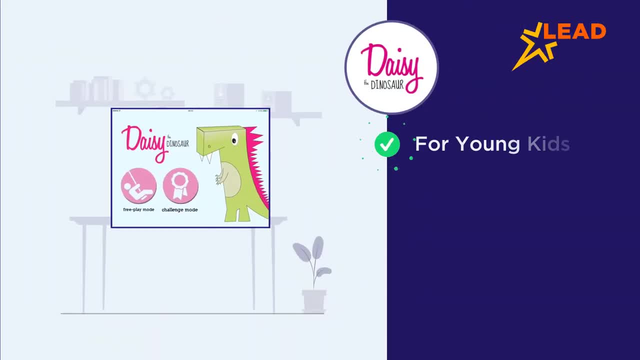 Daisy the Dinosaur is an app suitable for kids as young as 5.. As the name suggests, the game includes a cute dinosaur that can be programmed. Players use drag and drop commands such as turn, draw and shrink to control Daisy's movements. 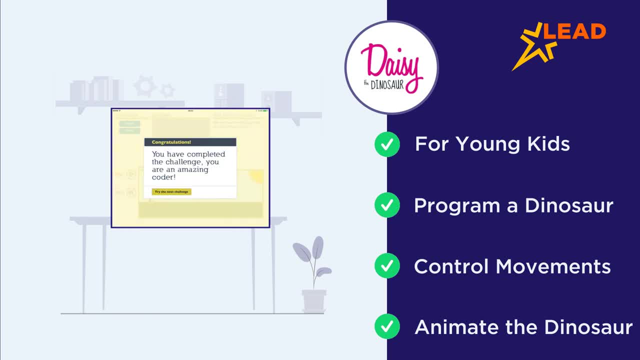 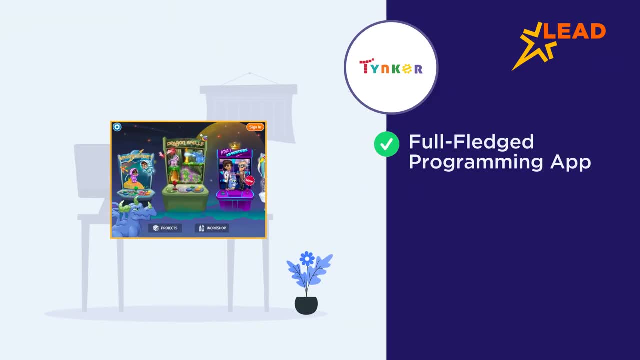 Animations such as jumping and dancing keep the kids engaged while they learn coding in the form of games. Tinker Tinker is a full-fledged programming app that has something for everyone, from novice to expert. The app starts with the fundamentals of coding, such as loops and sequences. 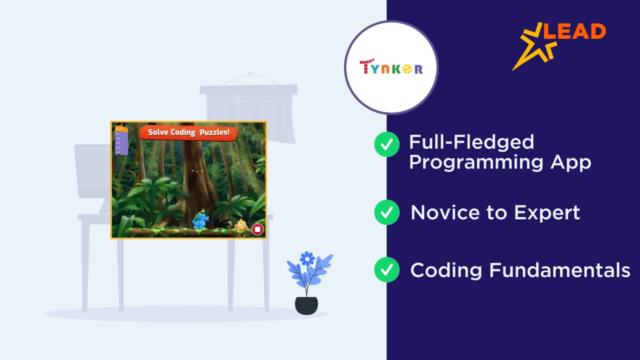 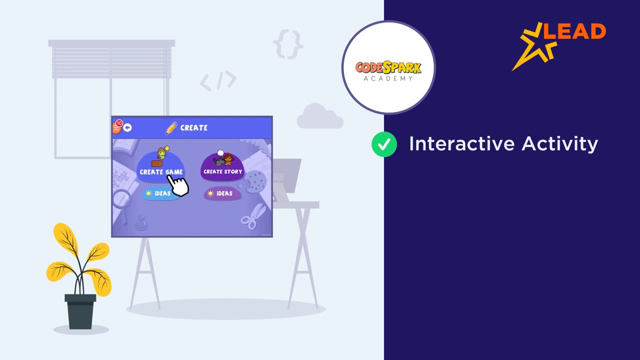 and then eases into real-world programming languages as kids spend more time on the app. As the app progresses, users learn how to design their own games using Python, JavaScript and other text-based programming languages. Codespark Academy. Codespark Academy turns coding into a fun, interactive activity that engages kids for hours. 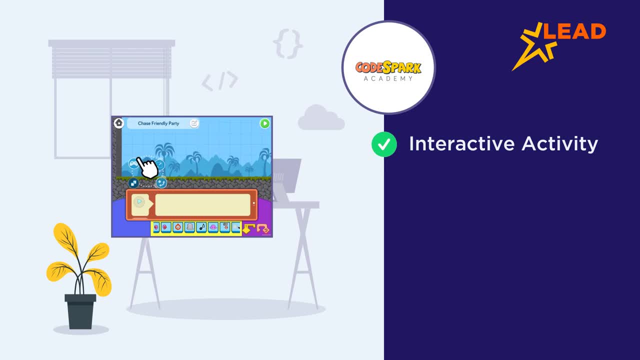 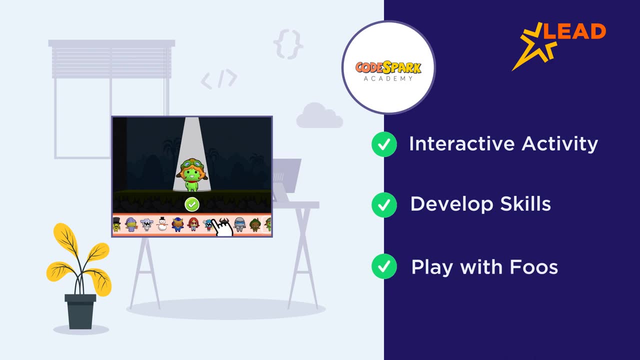 Through Codespark Academy, children not only learn programming but also develop logical thinking and programming. The app is the hint for kids to learn to solve problems by using the software. Codespark Academy is designed to help kids learn coding we use to improve their programming skills. 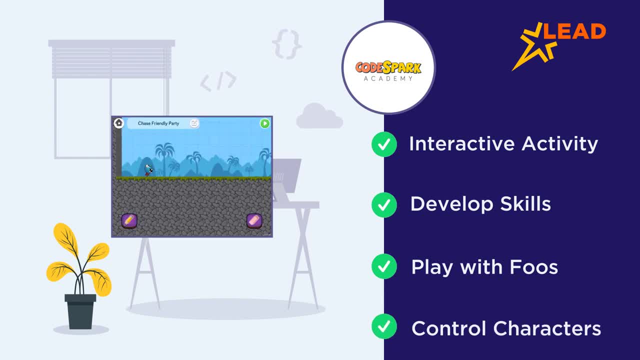 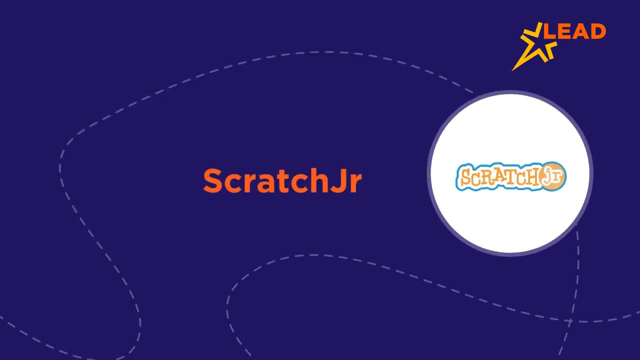 Adorable characters called Fuz take players on an adventure while teaching coding concepts Using sequencing and loops. players can control their characters to collect gems, donuts and other items. The game is divided into worlds that focus on different coding concepts: Scratch Junior. 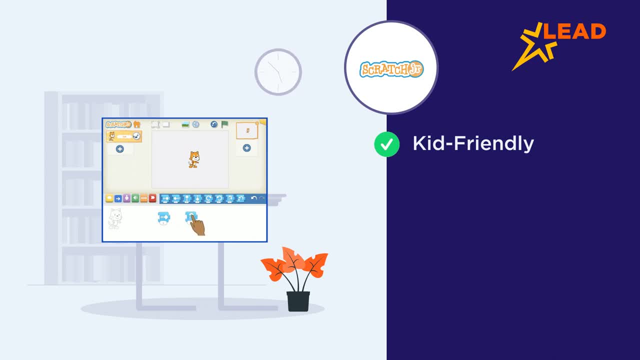 The kid-friendly version of the popular MIT Developed app Scratch Junior uses games and stories to build an interactive coding experience. Using word-free coding blocks, kids can control characters by instructing them to jump, dance and jump. Consisting of several allows kids to learn to play an active role. 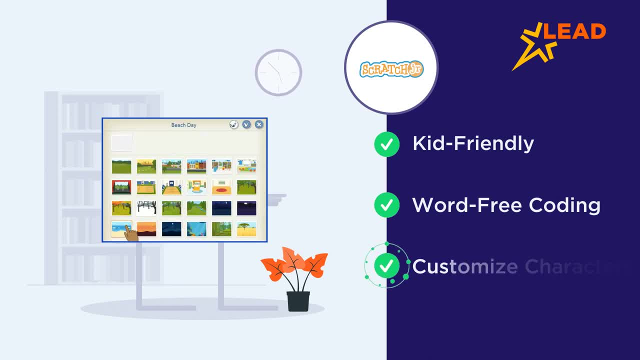 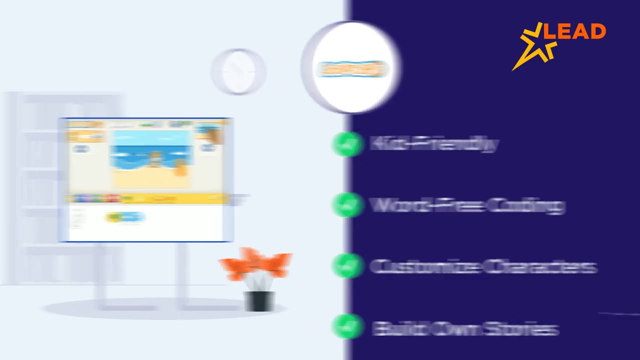 them to jump, move or even dance. All the characters are customizable, right from the color to the sounds. Kids can also use their own images and voices to personalize the characters. There are no particular goals, so children can explore and experiment with a wide range of coding blocks to build their own stories. 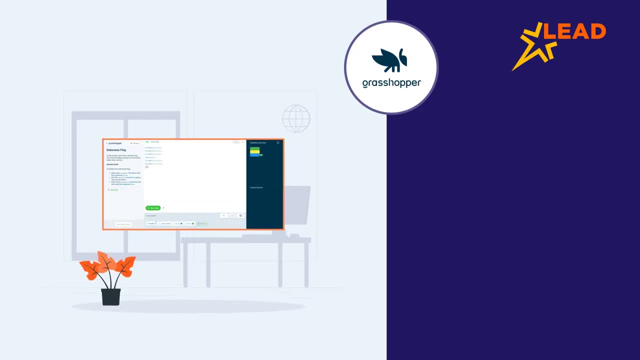 Grasshopper. Grasshopper is another coding app that focuses on both theory and practical coding, Developed by Google. the app is meant for older children who can grasp the knowledge of real-world coding. The app starts with a question gazing the user's experience level. Beginners are introduced to coding with. 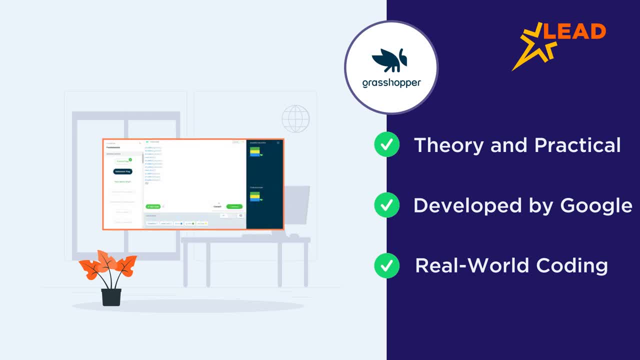 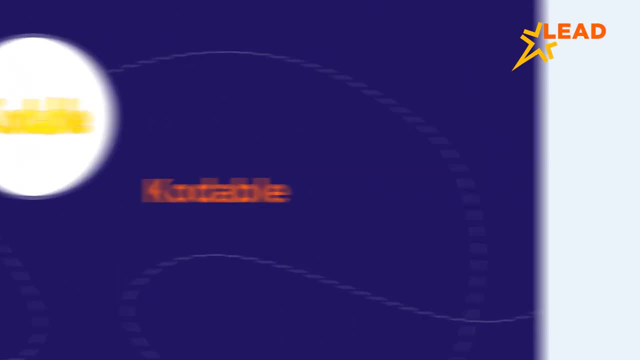 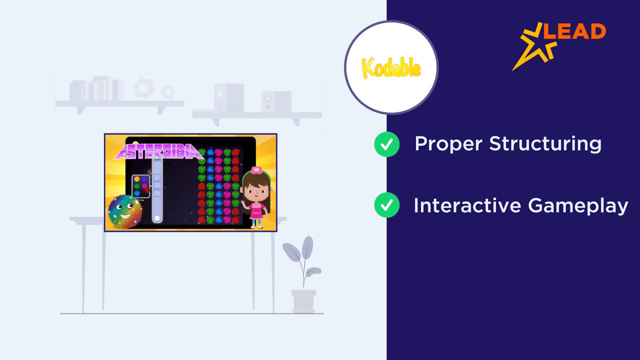 slides and short quizzes. Once kids master the theory, they can code puzzles that provide a hands-on experience Codable. Codable is an app that teaches multiple programming languages. with proper structuring, The interactive gameplay teaches kids the fundamentals of coding through kindergarten level and